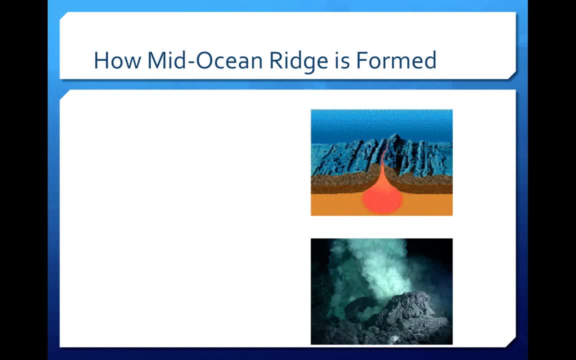 It's actually much different than I would have thought. Maybe you would have thought this is how it happens. So you have two tectonic plates And, like I said, we will talk more about tectonic plates, But just so you know now, tectonic plates are. 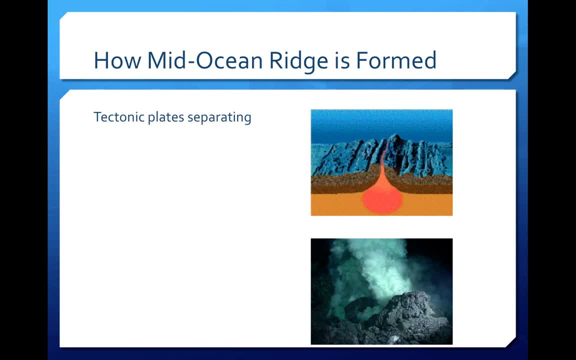 are the plates that the Earth's crust is made out of. So tectonic plates are the plates that the Earth's crust is made out of. So you would think- at least I would think- that mountains, or oftentimes mountains, are formed when those plates smash together. 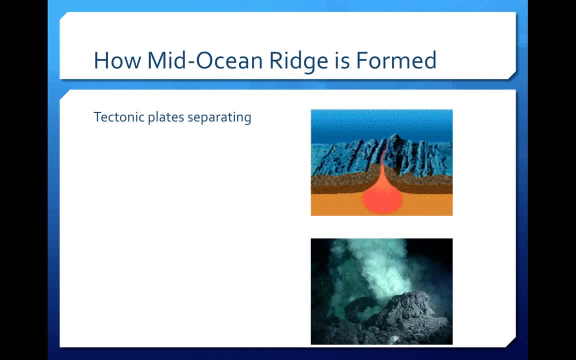 But actually mid-ocean ridge is formed when those tectonic plates separate. They go in opposite directions. So you can see right here. Okay, So we have one tectonic plate here, one tectonic plate here. 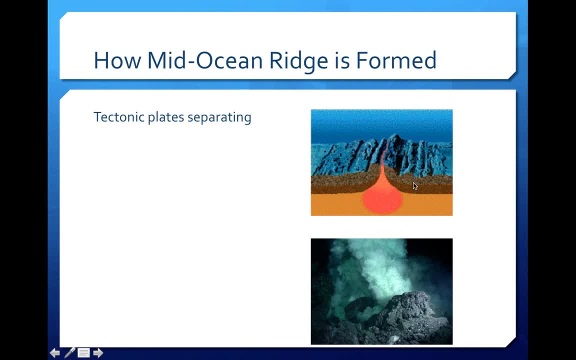 They're going in opposite directions. Okay, So if this tectonic plate is moving this way, if this tectonic plate is moving this way, then that creates a hole in the middle. Okay, And what does it look like is rising up from that hole? 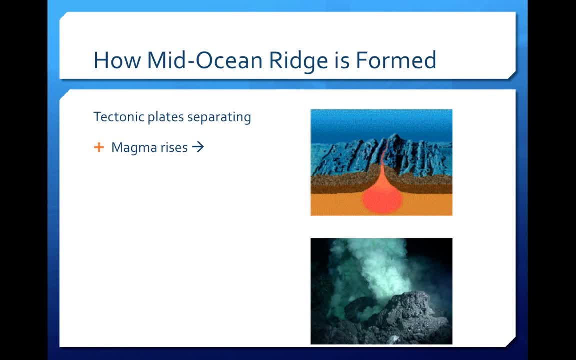 Right, Magma rises up. There's a whole bunch of magma right underneath Earth's surface. So that's going to. If two tectonic plates are opening up, you're going to create an opening to underground. There's a whole bunch of magma that's going to rise. 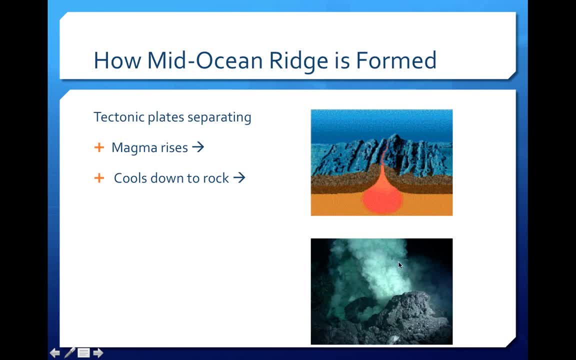 Okay. So when that magma rises, okay, so it's no longer under tectonic plates- it's going to be exposed to a bunch of water. So what do you think? What do you think is going to happen when that magma hits a bunch of water? 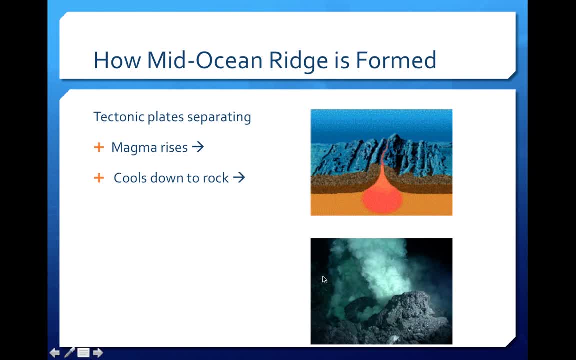 It's going to cool down And that's what you can see happening here. So what happens when the magma cools down? Right, It's going to form rock, It's going to turn hard And it's actually going to form mountains. 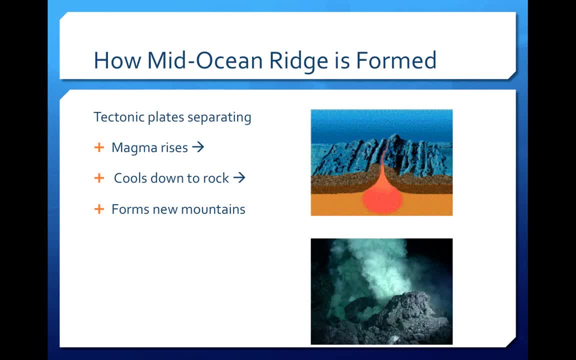 Okay, So what do we call rock that's formed when lava cools down? Right, We call that igneous rock, And that's what's forming the new mountains. So I want you to follow the computer mouse here, So this tectonic plate moving this way. 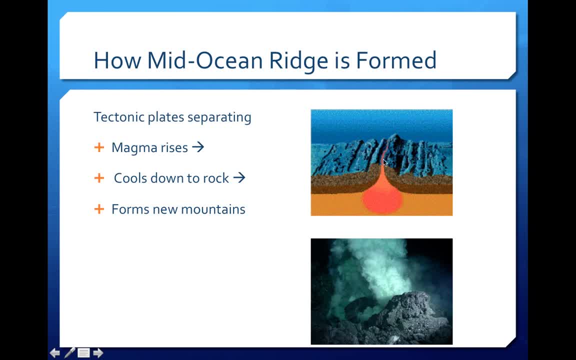 This tectonic plate. moving this way, They're separating from each other And as they do that, this magma keeps flowing up. This magma keeps flowing up, And when it hits the water it kind of instantly cools down and becomes hard rock. 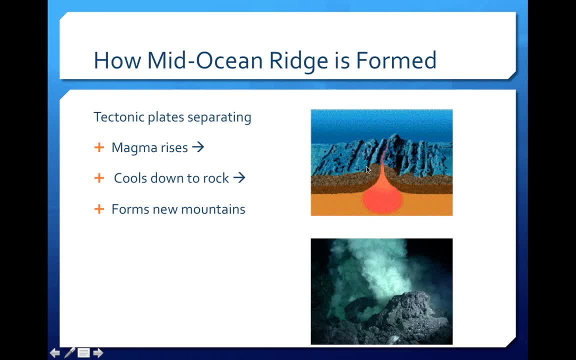 And that forms new, bigger mountains right in the middle here. Okay, So, and this is an important point, So if there's more and more new mountain being formed, let's take two positions on this mountain. Let's say, we're going to talk right in the middle here and way out on the edge over here. 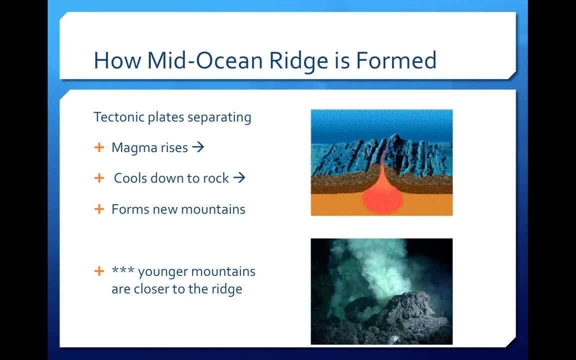 What's going to be the newest, youngest part of the mountain? Is it going to be right in the middle here, Or is it going to be on the edges over here? Right, This middle part is going to be the newest, youngest part of the mountain. 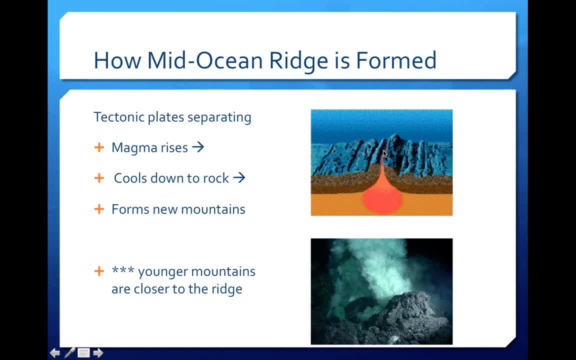 Because it was just magma, just like a couple seconds ago, Just barely cooled down, Just barely became that hard, igneous rock, Everything out here. it's been rock for a long time. Old news. It's been pushed out as those tectonic plates keep moving outwards. 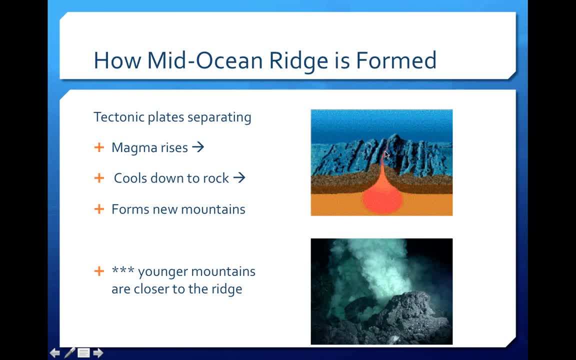 This is the old stuff. This is the good new stuff. Okay, That's how mid-ocean ridges are formed. Tectonic plates separate. The magma rises up from the middle and cools down and forms that new mountain rock, New igneous rock. 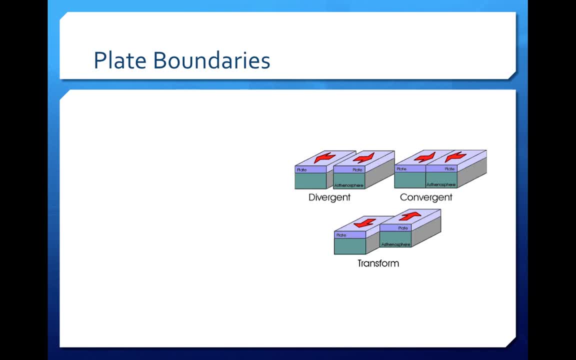 All right, So we're going to head back and just get a little bit of background on tectonic plates, How they move All this kind of stuff. Okay, So tectonic plates. There's three different type of ways that tectonic plates work on the Earth's surface. 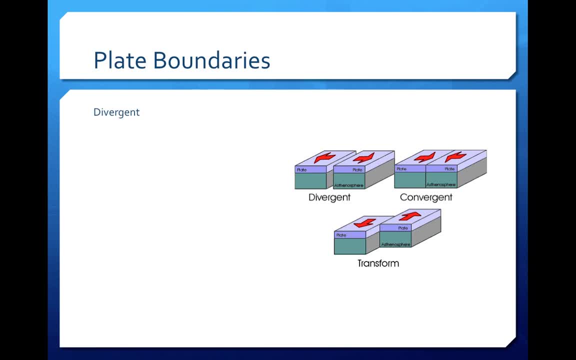 Okay, There's something called divergent plate boundaries. Okay, So, divergent plate boundaries. Here's a picture of it right here. What does it look like these two plates are doing? Okay, So the plates move away from each other. 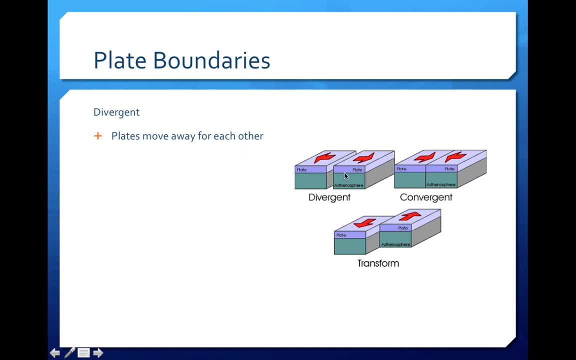 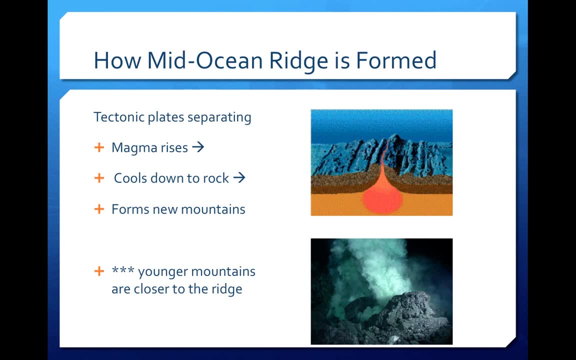 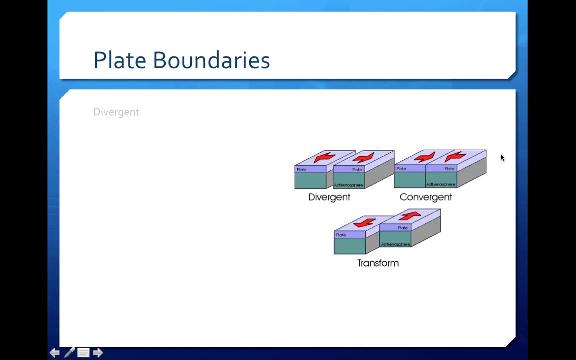 Okay, So tectonic plates are moving away from each other- Away from each other. So that's actually what's happening in a mid-ocean ridge: These tectonic plates are moving away from each other. They're a divergent plate boundary. 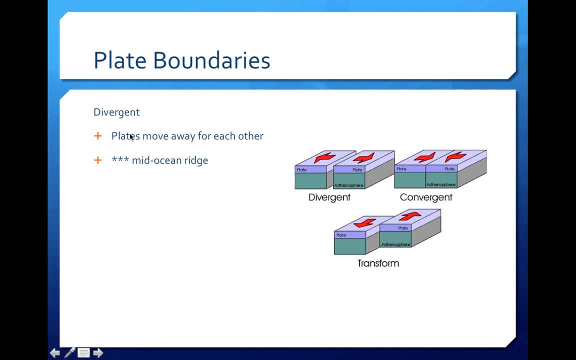 Okay, Exactly, A mid-ocean ridge is a divergent plate boundary. Okay, Convergent plate boundary, Convergent plate boundary. So what does it look like? is happening here if we look at the arrows? Okay, These tectonic plates. 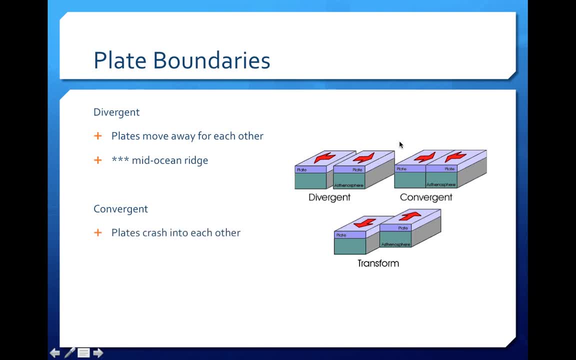 These tectonic plates actually crash into each other. It's the opposite of divergent: These tectonic plates are crashing into each other. So this is actually usually how mountains are formed on land: Two plates crashing into each other kind of builds up a big mountain here in the middle. 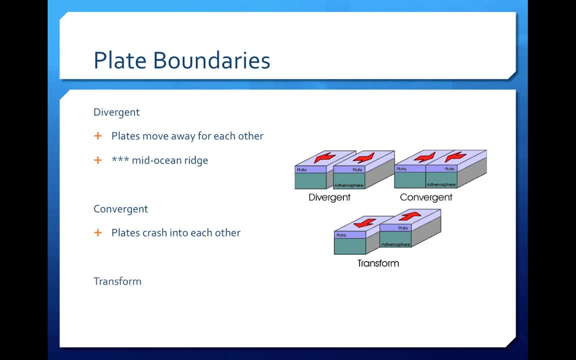 All right, And there's one more type of plate boundary. It's called a transform plate boundary. It's called a transform plate boundary, And so it's different. It's not moving away from each other, It's not crashing into each other. 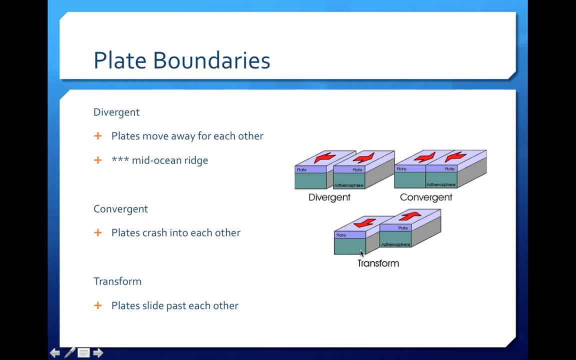 It's actually just moving side by side And this is actually a lot of places where earthquakes occur. So, like San Andres that movie, There's something called the San Andres fault line in California. This is what happens there. They're just sliding past each other, which can cause massive earthquakes. 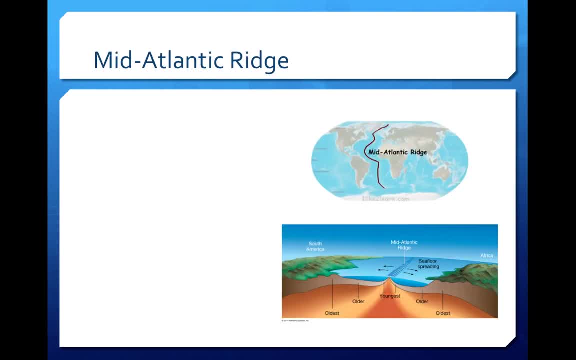 All right, And so, finally, finally, we talked about mid-ocean ridges, how they're formed, different plate boundaries, So something important that you need to know about is the mid-Atlantic ridge. Okay, So there's this specific thing called the mid-Atlantic ridge. 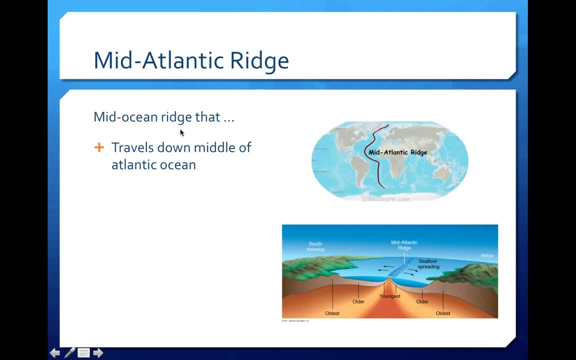 So it's a mid-ocean ridge, which is again, if we go back to the very beginning, it is an underwater mountain range, And it travels down the middle of the Atlantic Ocean. See, you can see it right here. 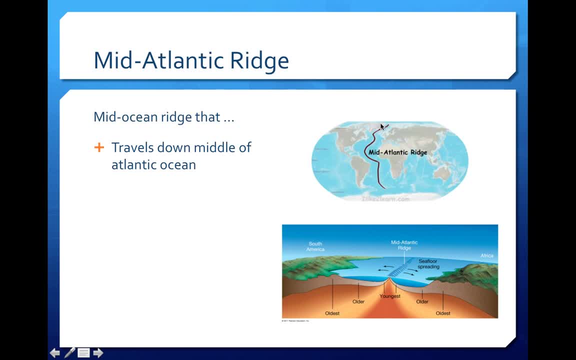 So, basically, the mid-Atlantic ridge is the biggest, most famous, most important mid-ocean ridge in the entire world. It goes- look at how big it is- It goes through the entire planet. Okay, So it starts way up here near the North Pole, goes past America. 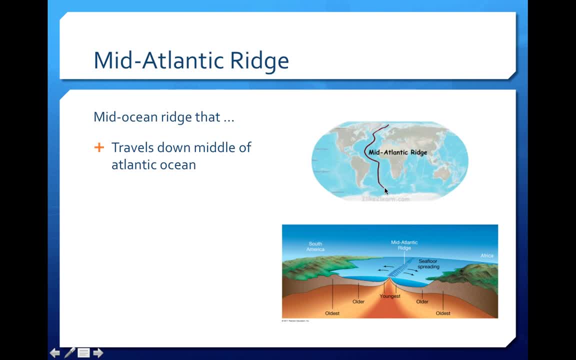 Past Mexico, past Africa and South America. It goes all the way down to the South Pole. So that's a huge mid-ocean ridge. And it's called the mid-Atlantic ridge because? why? Because it goes right through the Atlantic Ocean. 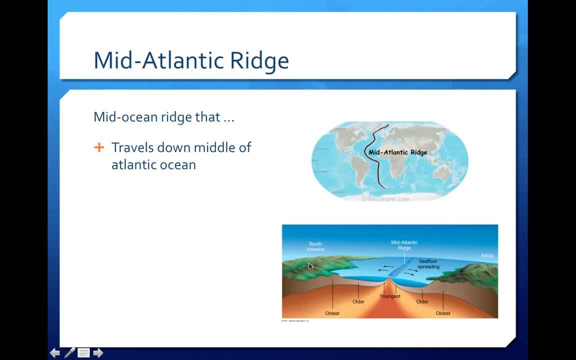 Okay, here's a picture of the mid-Atlantic ridge. You can see South America's on one side, which would be right here- Africa's on another side, You can see right here. This is also a really good picture. This is a picture of just showing how that mid-Atlantic ridge is formed. 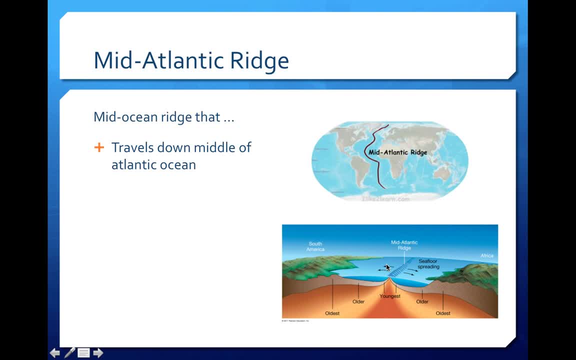 Again, you can see the two tectonic plates. Are they going towards each other or away from each other? Right, they're going away from each other And, as we know, okay, as they move away, what's going to bubble up here in the middle? 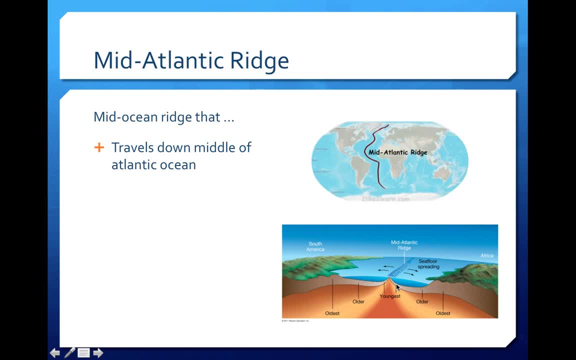 Magma, And as soon as that magma hits the water it's going to cool down, Okay, form new rock. So the newest, youngest Rock part of the mountain is going to be right in the middle And the old stuff's going to be pushed away. 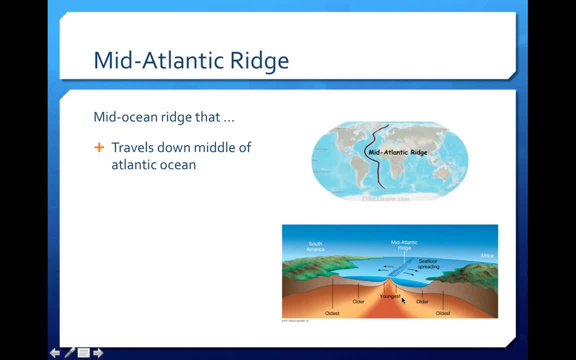 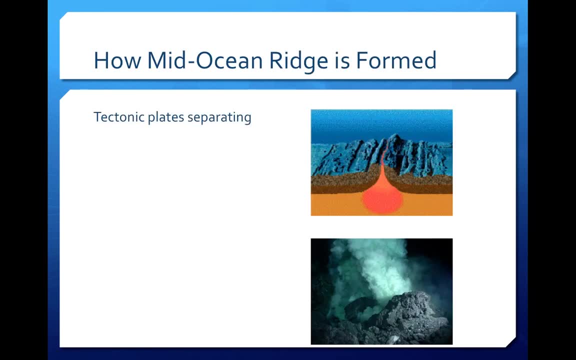 Pushed away. Oldest you can see is right here. Alright, awesome job you guys. Just a quick, quick review. So we went over. We went over what is a mid-ocean ridge? It's an underwater mountain range. 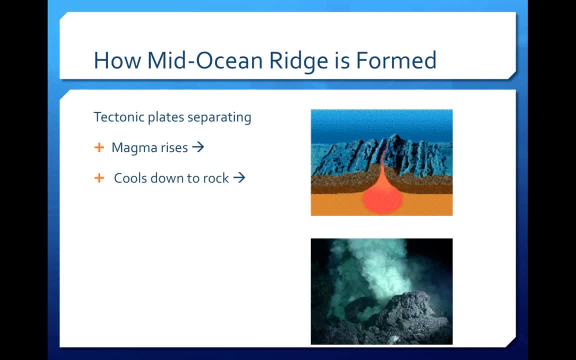 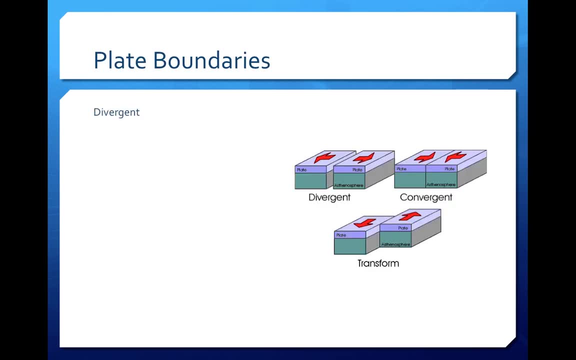 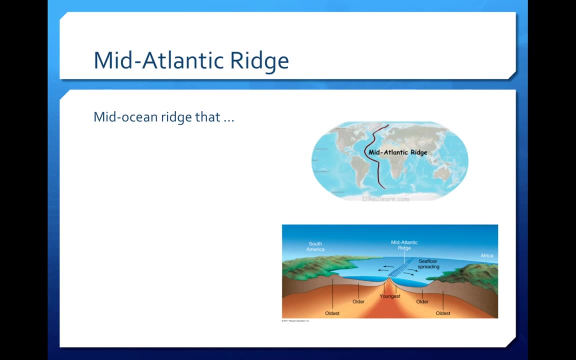 We went over how they're formed by tectonic plates moving away from each other, Magma rises up and cools down- Learned about the different plate boundaries- divergent, convergent and transform. And learned about the most important, most famous mid-ocean ridge called the mid-Atlantic ridge. 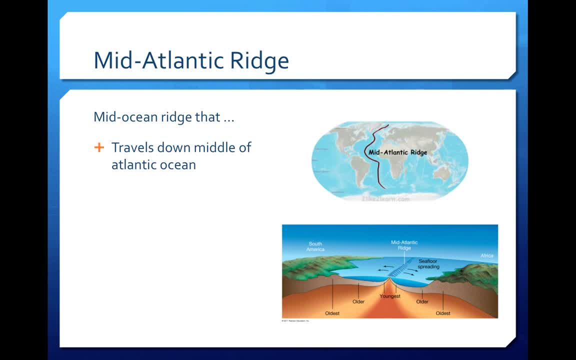 running through the Atlantic Ocean. Alright, awesome job you guys.